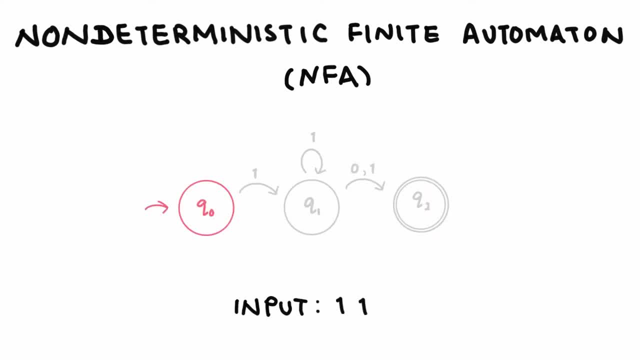 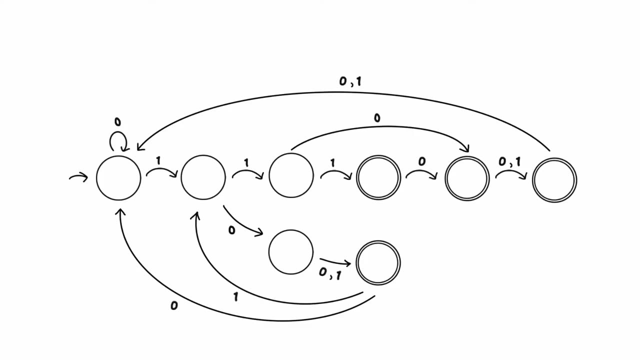 unlike DFAs, for every symbol in the input, the next state to transition into is not always determined. There can be zero or more than one state that the machine could choose to transition into. For example, this is a DFA, which we will call M, that accepts any string that contains a. 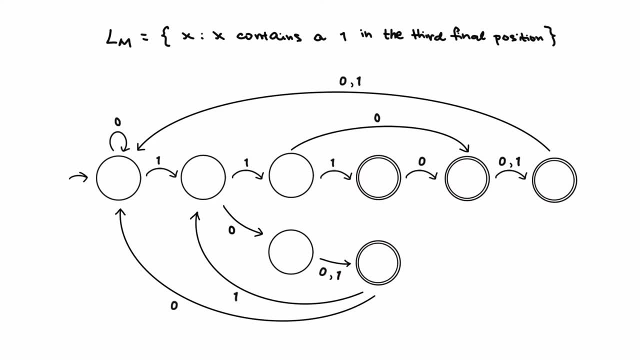 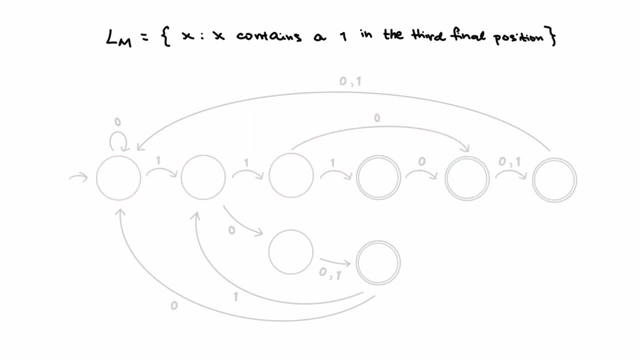 1 1 0 0,, but it rejects 1 0 0 0 and 1 0 1 1.. The NFA that recognizes the same language will be as simple as this. Notice how, when a 1 is encountered, Q0 can choose to remain in Q0, or it could. 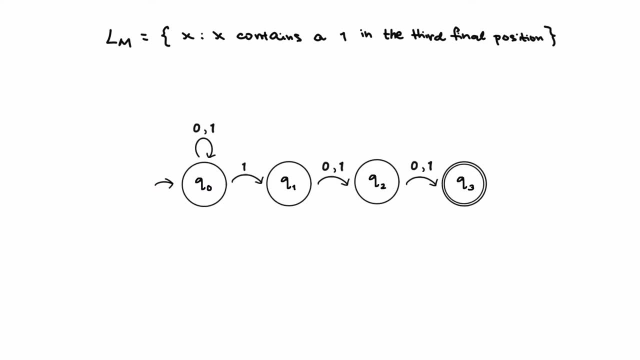 transition into Q1.. There are also no arrows coming out of the accept state Q3. However, like the DFA, it still accepts 1 1- 1 and it also accepts 1 1 0- 0.. You might have noticed how it also could have. 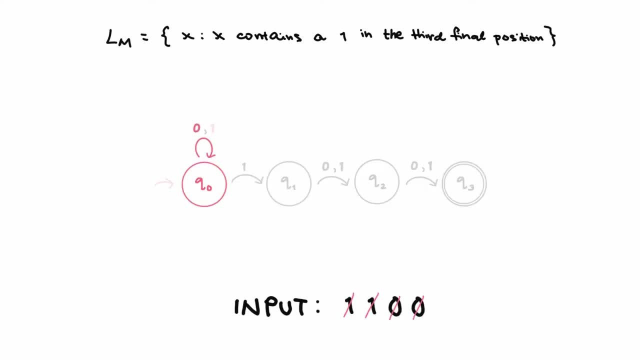 rejected 1 1 1 and 1 1 0 0 by choosing to remain in Q0 the entire time. And you aren't wrong. However, the NFA accepts a string as long as there is at least one path to an accept state. 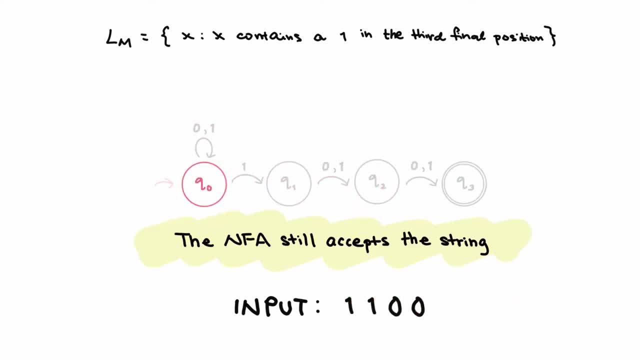 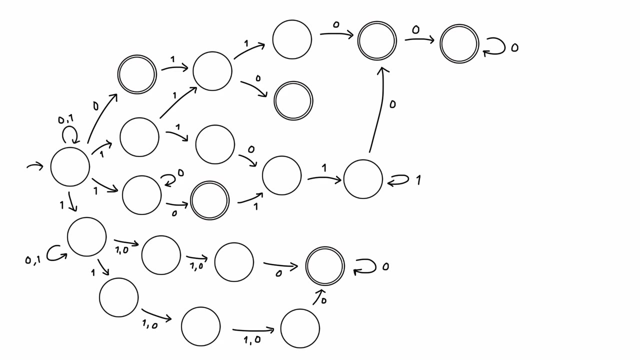 So, although there is a path that would reject the string, the NFA still accepts the string because there is another path to an accept state. Let's look at another example to better understand how an NFA accepts the string. Consider this NFA: By construction, this NFA would accept. 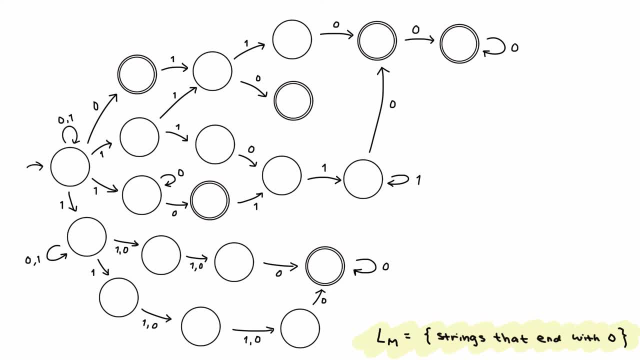 any string that ends with a 0 and will never accept the string that ends with a 1.. So, on an example input 1 0, 0, it could take this path, or this path and accept the string. or it could take this path and accept the string, or it could take this path and accept the string. 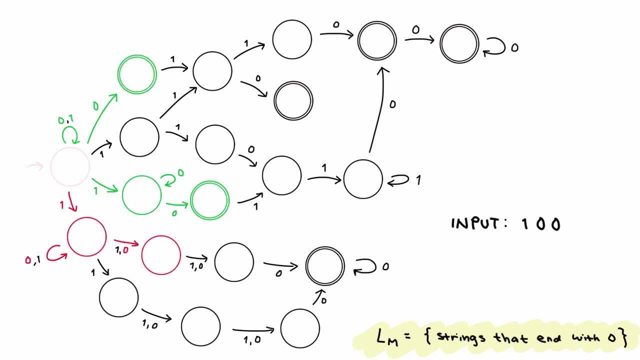 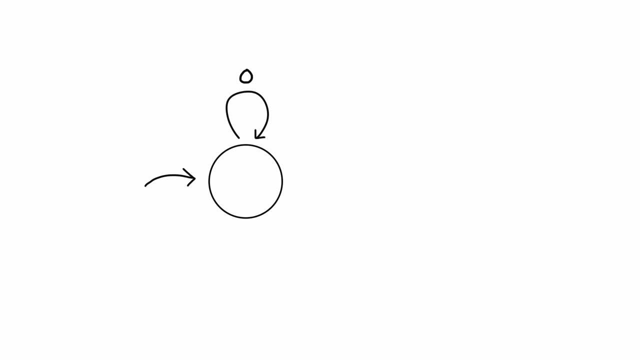 or it could take this path and reject the string. However, it doesn't matter which path the NFA decides to take. As long as there exists one path that causes the machine to end in an accept state, then we say the NFA accepts the string. Additionally, NFAs can also transition on the. 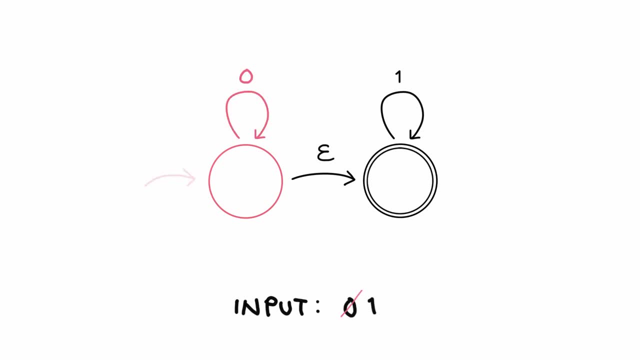 empty string. When an NFA chooses to transition on the empty string, no symbol from the input string is consumed. So, going back to the example, if you choose to take a string that ends with a 0, and So going back to our first NFA that accepts all strings containing a 1 in the third, final position, 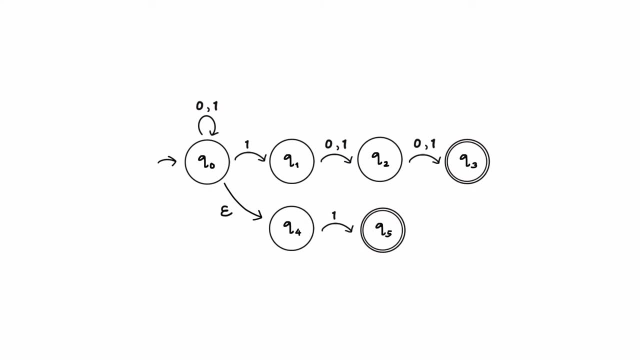 let's add these two new states with an empty transition. The NFA now accepts all strings containing a 1 in the third final position, or it also accepts the single 1.. What we have been looking at is the state diagram of an NFA. 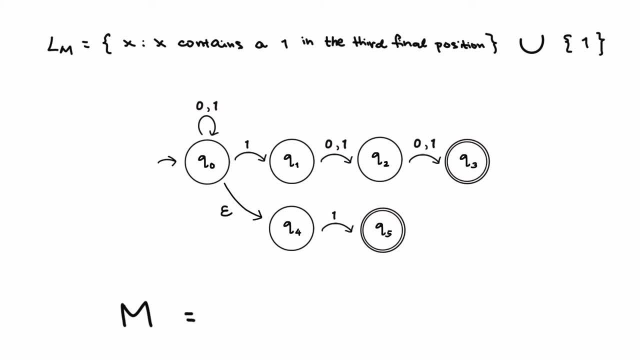 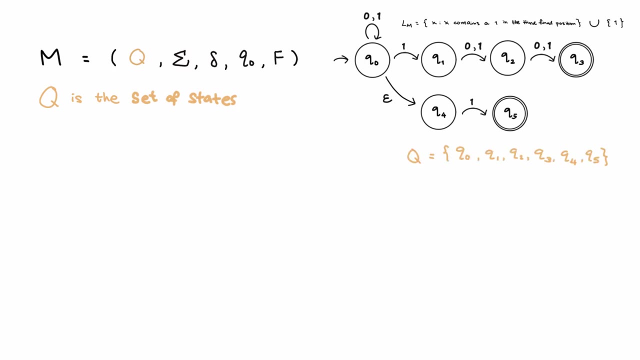 And, like DFAs, NFAs are also 5-tuples. when formally defined, Q is the finite set of the machine states. So for our previous NFA that would be the set containing Q0,, Q1,, Q2, Q3, Q4, and Q5. 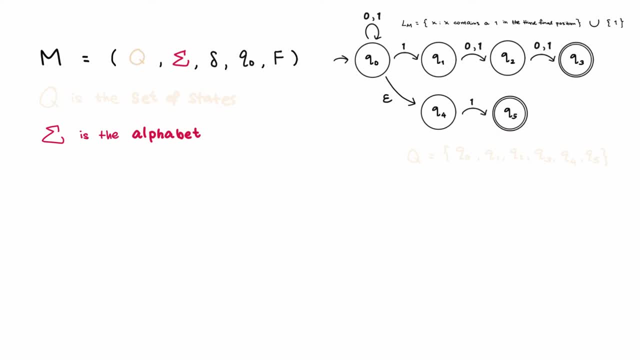 Sigma is a finite set called the alphabet, which is all the symbols recognized by the automaton, So in this case it is the set containing 1 and 0.. Delta is the transition function And because NFAs can transition on the empty string. 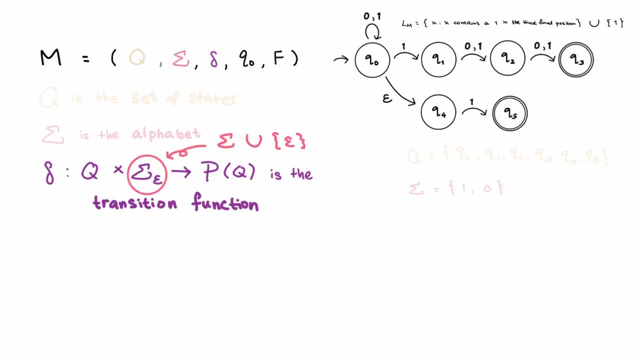 this symbol here represents everything recognized by the NFA, along with the empty string, And because NFAs can have 0 or several choices to transition into, the transition function gives us a set of possible states instead of just a single state, And that's what this P symbol here represents. 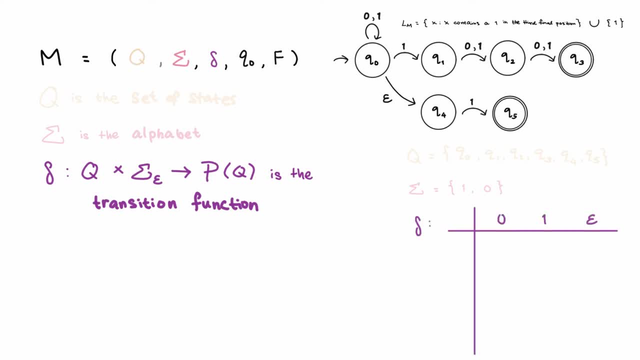 So, going back to our NFA, the transition function is defined like so: Q0 will remain in Q0 on a 0. And on a 1, it can choose to remain in Q0 or transition into Q1. Or it could empty, hop over to Q4. 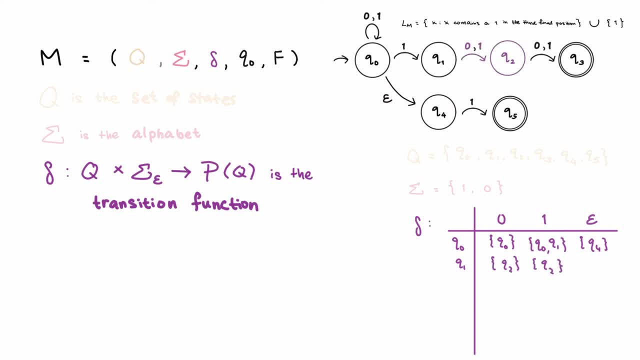 Q1 can only transition into Q2 on a 0 and 1.. Q2 can also only transition into Q3 on a 0 and 1.. And Q4 transitions into Q5 on a 1.. Finally, for the states and symbols that have no transitions: